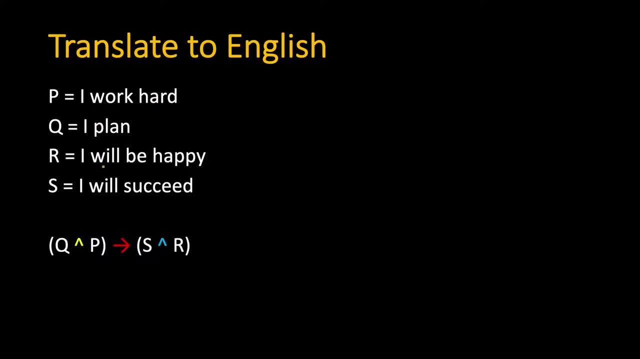 convert it to one meaningful English sentence. and the second one is converting back from the English translation to a formula. So first let's see how we can convert this propositional formula to an English sentence. So we see, here there is one implication. So it means that somewhere there 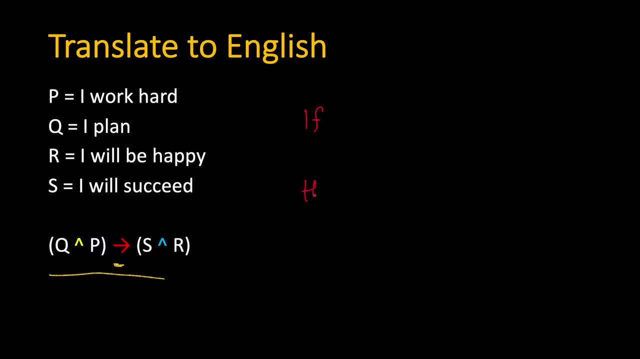 will be one. if and there will be one, then Now we have to fill this part, these two parts, So this is done. Next, we have Q and P. So Q is I plan. So if I plan, then we have this, and So we have. and. 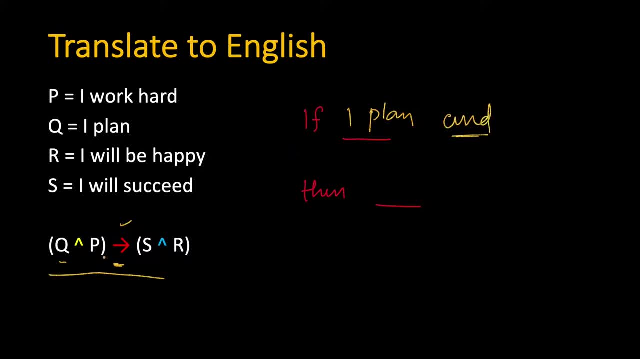 So P is I work hard, If I plan and I work hard, then then after then we will find: what is this part? So this part is S and R. So what is S? S is I will succeed, And then we will write and for this, this connector, and then R, So R is I will be happy. 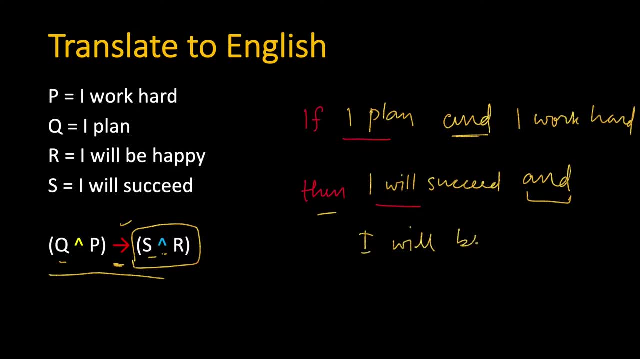 And then we will write: and for this, this connector, and then R, So R is I will be happy. So this propositional formula translates into this English sentence: If I plan and I work hard, then I will succeed and I will be happy. Now let's try the other way. 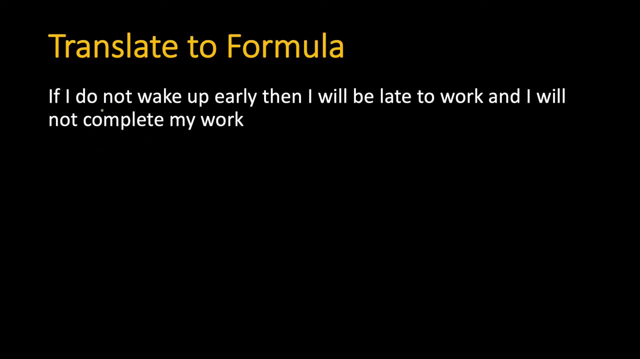 So let's say we are given this English sentence: If I do not wake up early, then I will be late to work and I will not complete my work. So let's first find out what are the connectors. So let's first find out what are the connectors. So let's first find out what are the. 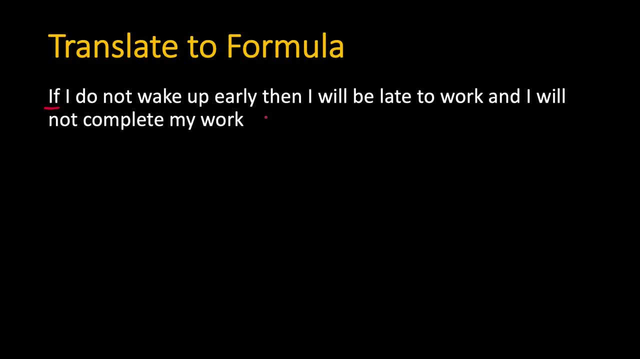 connectors. So we see here if, If, and then we see here. So we know that there will be one implication here and there will be something here and something in this part, So let's find out the remaining. So this whatever sentence is after then will come here and whatever is between if. 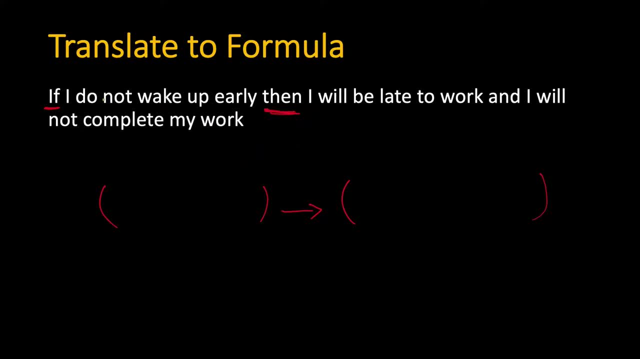 and then will come here. So let's see further. I do not wake up, So we see here not. So let's write this not. And I do wake up, So let's write the propositions. So it's here. I do wake up early. 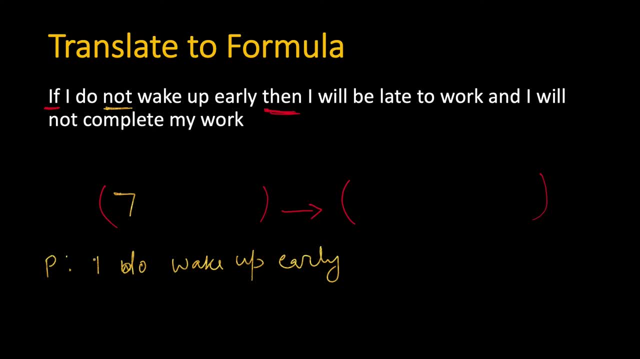 So generally we write the propositions in affirmative way. So we could have thought that why don't take this complete thing I do not wake up early as one proposition. So here not is a connector and generally we write the propositions in whatever is affirmative and not negative things. So P is here and this negation of this will be: I do not wake. 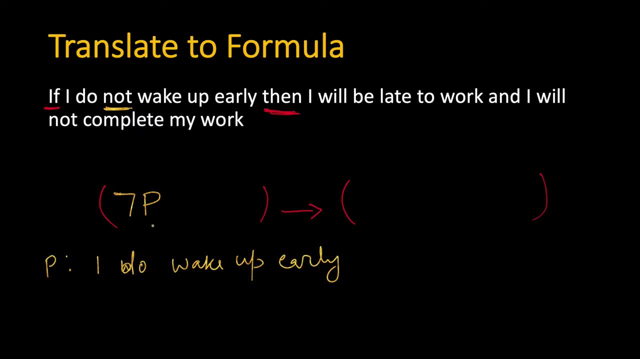 up early, So we have this part is complete. there is nothing else here. Then the second sentence is: I will be late to work, So let Q is. I will be late to work, So write Q here. and then we have AND, So AND is another connector, so write this. I will not complete my work. 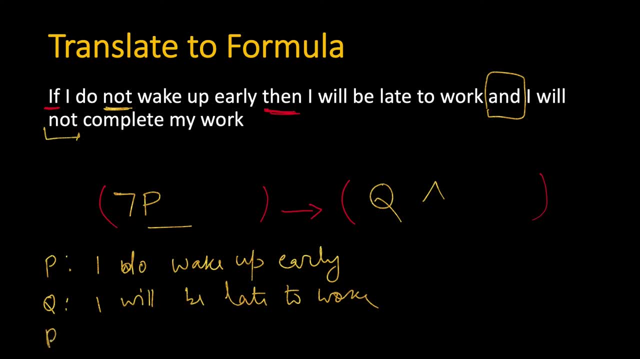 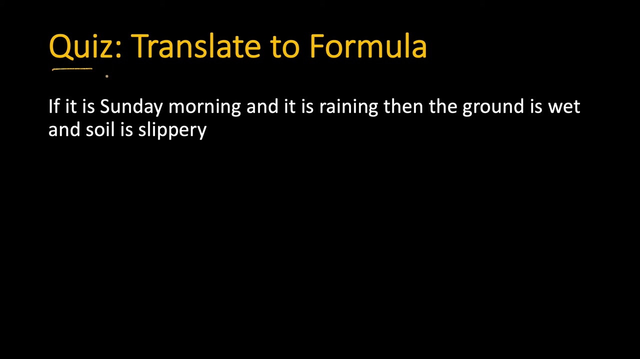 So again, not is a connector. So R is: I will complete my work. So Q is not complete my complete my work, and not of that will be this. So the formula for this would be this one: not P implies Q and not R. So now let's practice with one more example. So we are given here: 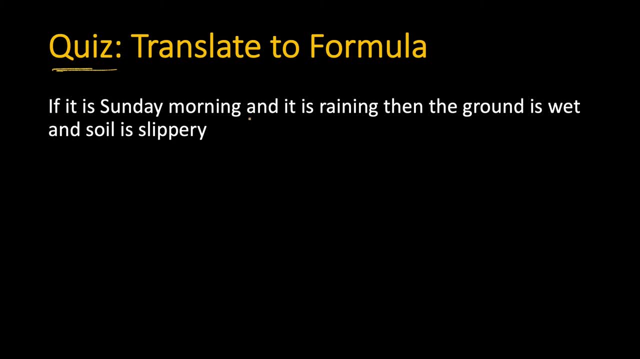 English sentence: if it is Sunday morning and it is raining, then the ground is wet and soil is slippery. So please try out this example and try to convert it to one formula- propositional formula- and post your answer in the comment section. So thanks for watching. See you in the next video.